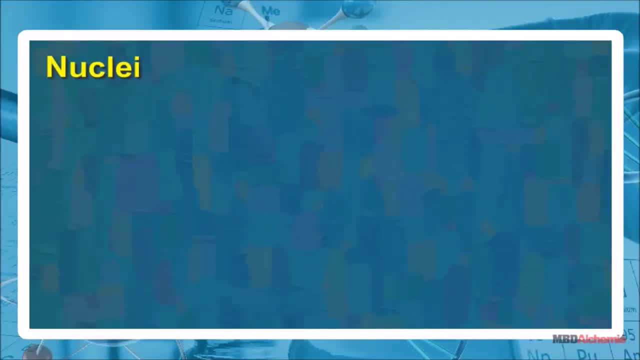 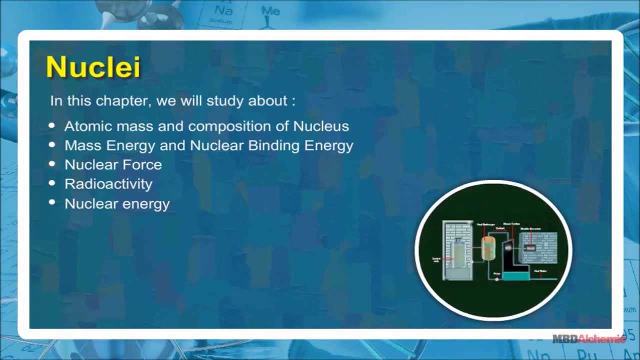 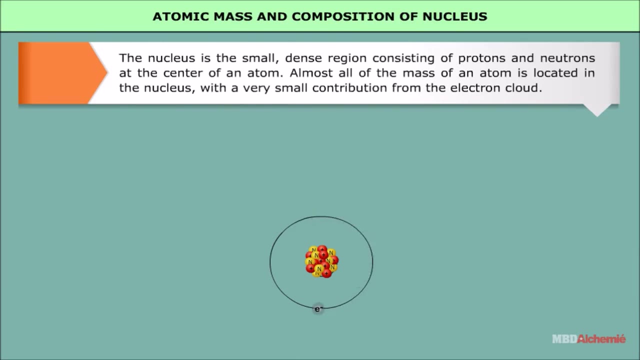 atomic mass and composition of nucleus. the nucleus is the small, dense region consisting of protons and neutrons at the center of an atom. almost all of the mass of an atom is located in the nucleus, with a very small contribution from the electron cloud. protons and neutrons are bound together to 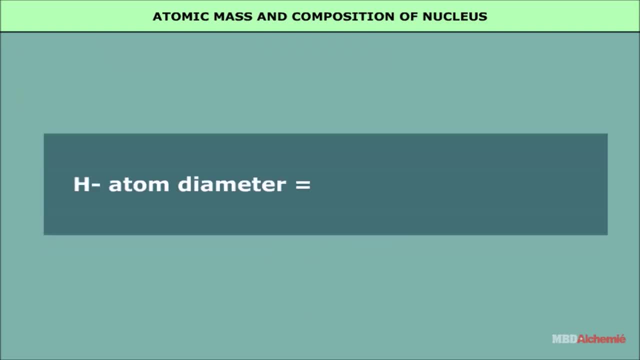 form a nucleus by the nuclear force. the diameter of the nucleus is in the range of 1.75 Fermi for hydrogen- the diameter of a single proton- to about 15 Fermi for the heaviest atoms, such as uranium. these dimensions are much smaller than the diameter of the atom itself: the masses of an. 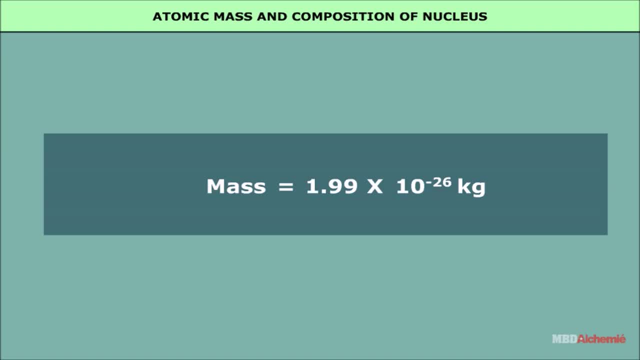 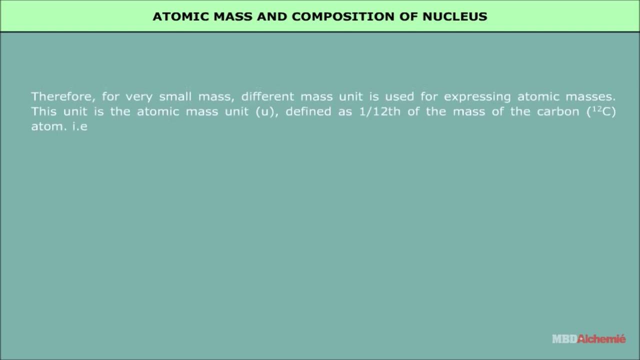 atom and its nucleus are very small as compared to a kilogram, for example, mass of a carbon atom is one point nine, nine, two, six, four, seven into ten, raised to power minus 26 kilogram. therefore, for very small mass, different mass unit is used for expressing atomic masses. This unit, 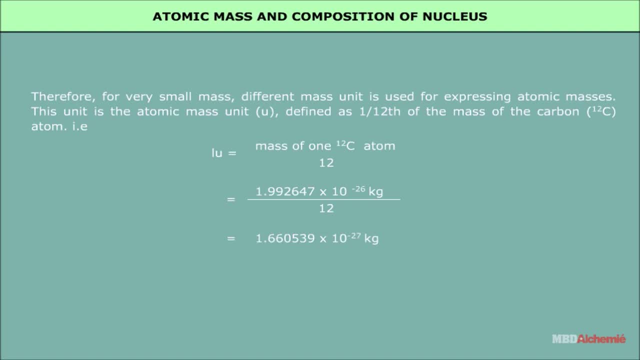 is the atomic mass unit defined as 1 by 12 of the mass of the carbon atom, That is, 1U is equal to mass of 1. 12 carbon atom divided by 12 is equal to 1.660539 into 10 raised. 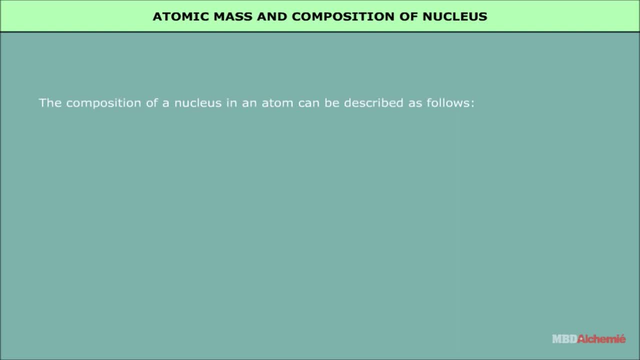 to power minus 27.. The composition of a nucleus in an atom can be described as follows: Z. atomic number is equal to number of protons, N. neutron number is equal to number of neutrons. A mass number is equal to Z plus N- total number of proton and neutrons. Here some important 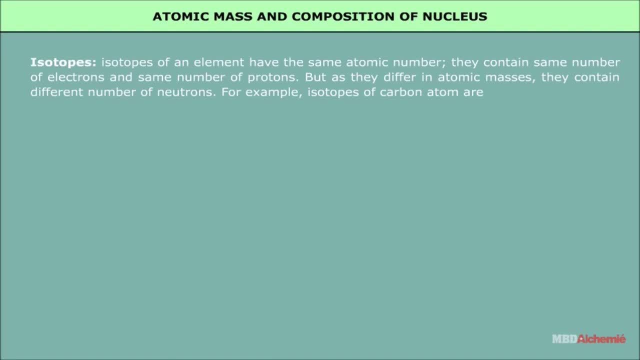 points are isotopes. Isotopes of an element have the same atomic number. They contain same number of electrons and same number of protons, But as they differ in atomic masses, they contain different number of neutrons. For example, isotopes of carbon atom are isobar. Isobars have same mass number. 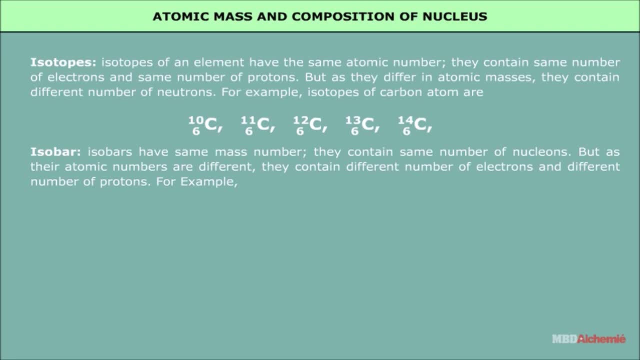 They contain same number of nucleons But as they are atomic, they contain same number of neutrons. For example, isotopes of carbon atom are isotonic. How many neutrons are isotonic? If the atomic numbers are different, they contain different number of electrons and different. 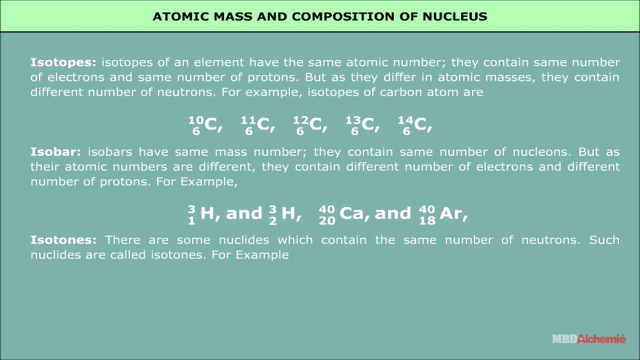 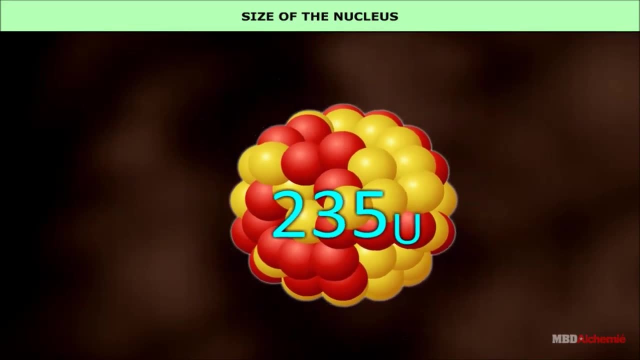 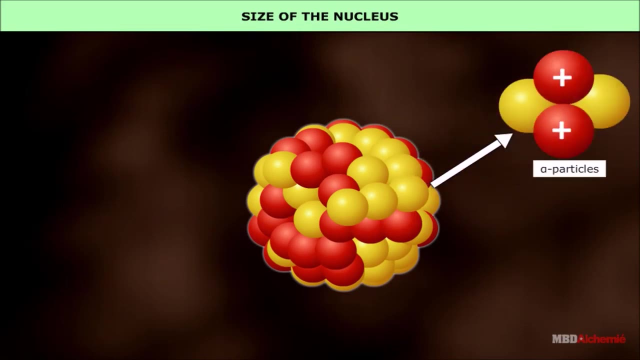 number of protons, For example isotones. There are some nucleides which contain the same number of neutrons. Such nucleides are called isotones. For example: size of the of. alpha particles are projectiles that bombard targets made up of various elements. the sizes: 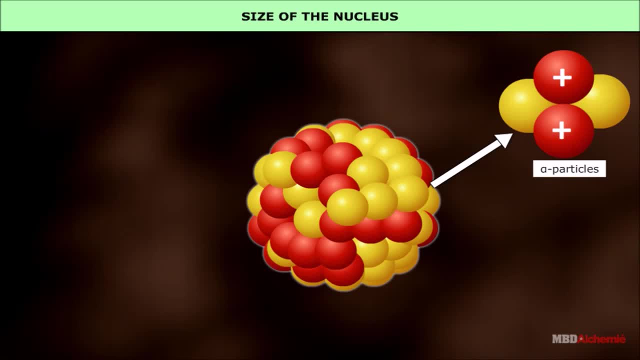 of nuclei of various elements have been accurately measured. It has been found that a nucleus of mass number A has a radius r is equal to r0, A raised to power 1 by 3, where r0 is equal to 1.2 into. 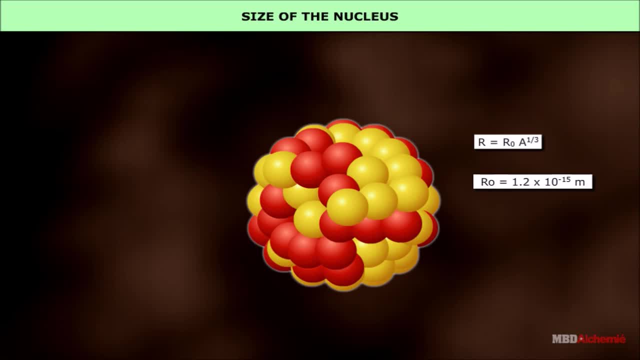 10 raised to power minus 15 meter. This means the volume of the nucleus, which is proportional to r cube, is proportional to A. Thus the density of nucleus is a constant independent of A. for all nuclei The density of nuclear matter is approximately 2.3 into 10 raised to power, 17. 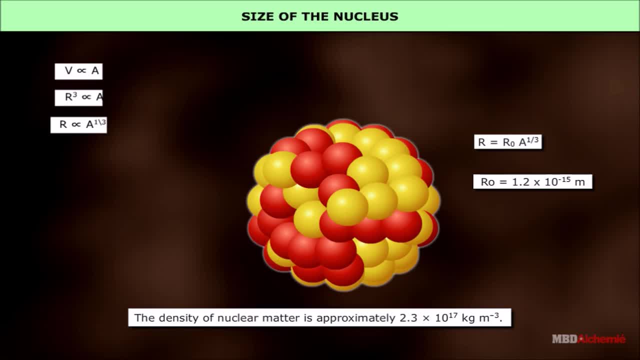 kilogram per meter cube. This density is very important, Very large compared to ordinary matter. say water, which is 10 raised to power, 3 kilogram power minus 3..